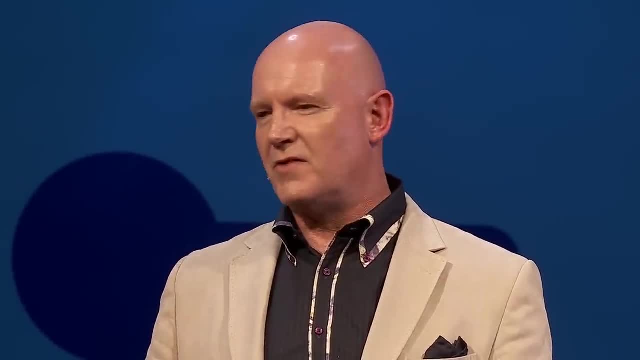 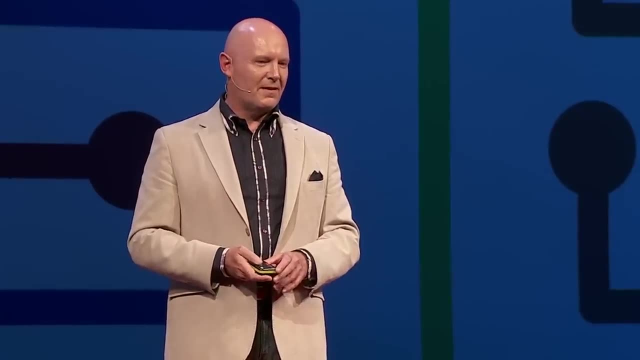 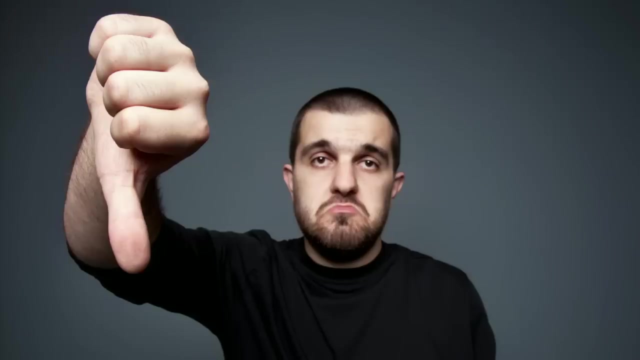 day. I said to her it's October the 1st today, and she said: I know, isn't it dreadful? It's hard to when somebody's that negative And another form of negativity, complaining. Well, this is the national art of the UK, It's our national sport. We complain about the weather, about sport. 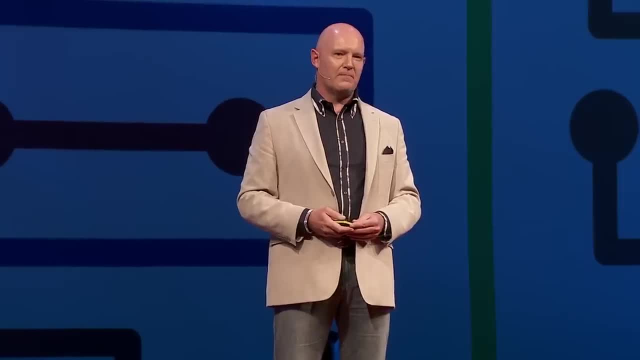 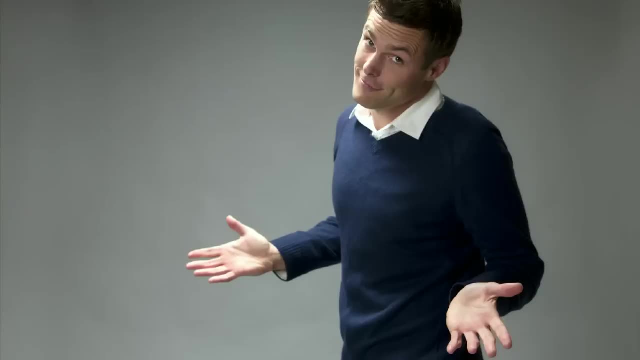 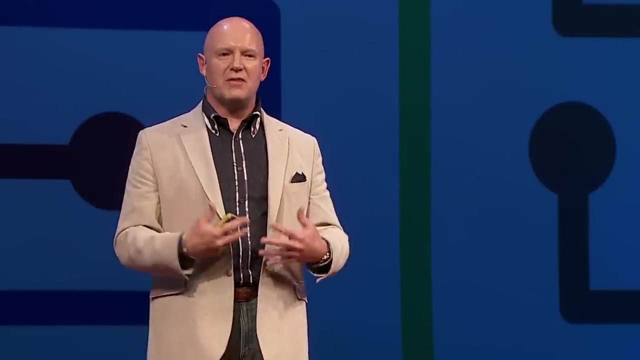 about politics, about everything, but actually complaining is viral misery. It's not spreading sunshine and lightness in the world. Excuses: We've all met this guy. Maybe we've all been this guy. Some people have a blame thrower. They just pass it on to everybody else and don't. 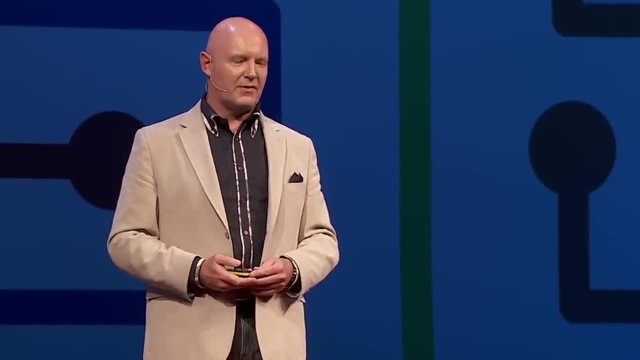 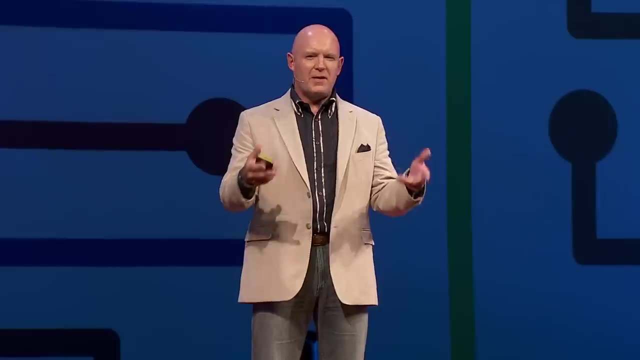 take responsibility for their actions. And again, hard to listen to somebody who's being like that. Penultimate, the six of the seven. embroidery exaggeration. It demeans our language actually sometimes. For example, if I see something that really is awesome, what do I call? 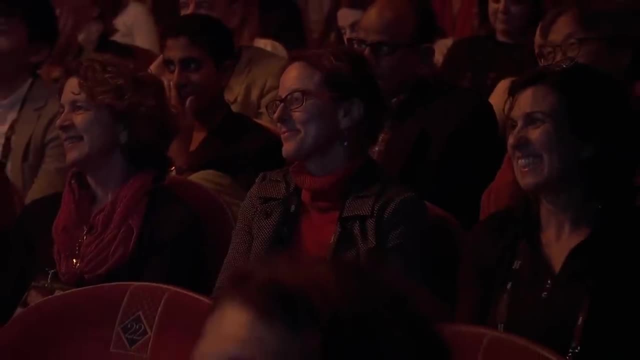 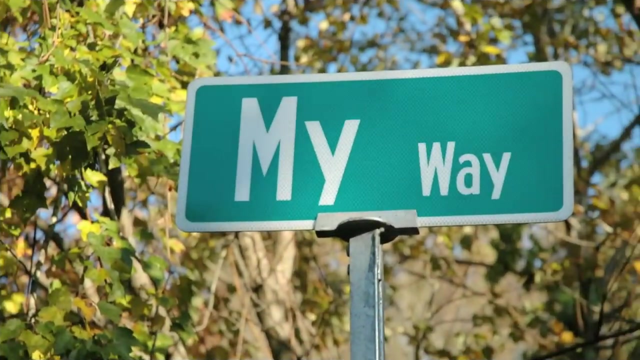 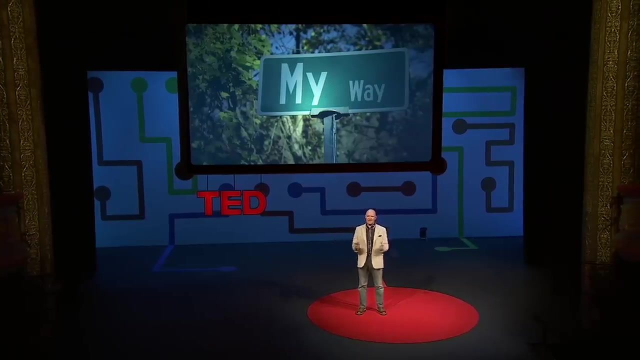 it. And then, of course, this exaggeration becomes lying, out and out lying, and we don't want to listen to people we know are lying to us. And finally, dogmatism, The confusion of facts with opinions, When those two things get conflated. you're listening into the wind. 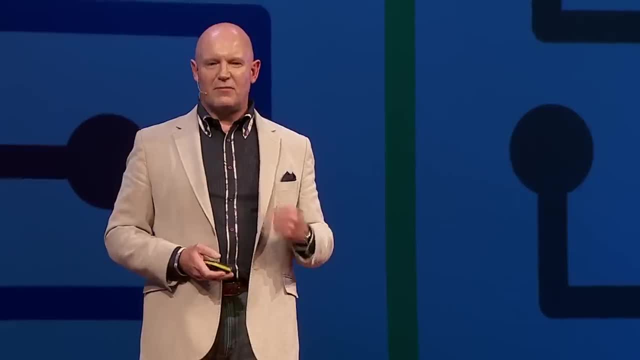 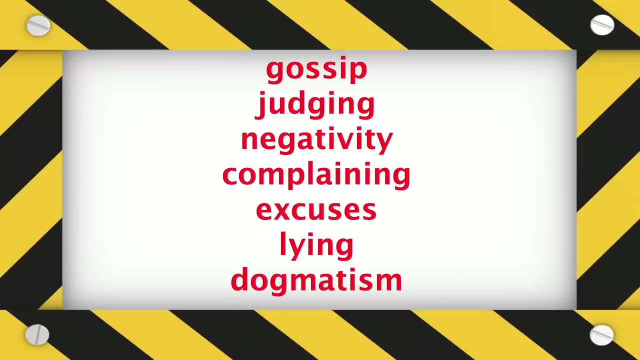 You know, somebody is bombarding you with their opinions as if they were true. It's difficult to listen to that. So here they are: seven deadly sins of speaking. These are things I think we need to avoid. But is there a positive way to think about this? Yes, there is. I'd like to. 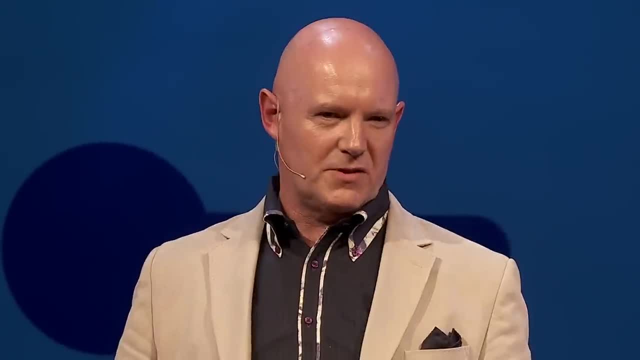 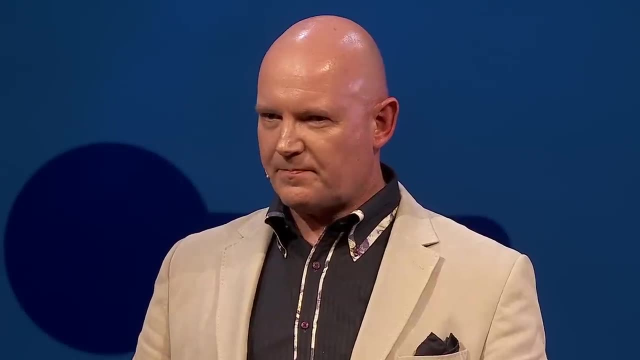 suggest that there are four really powerful cornerstones, foundations that we can stand on if we want our speech to be a reality. And I think that's the first thing we need to do, And I think that's the second thing we need to do, And I think that's the third thing we need to do To be 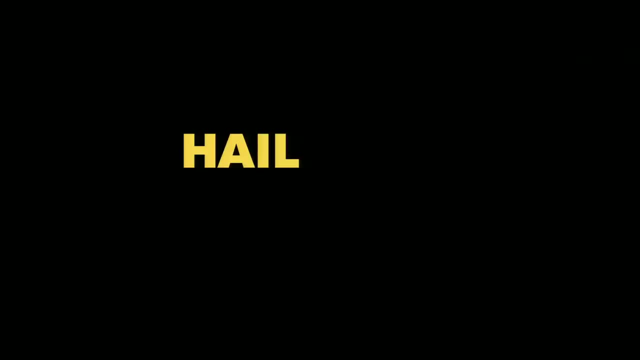 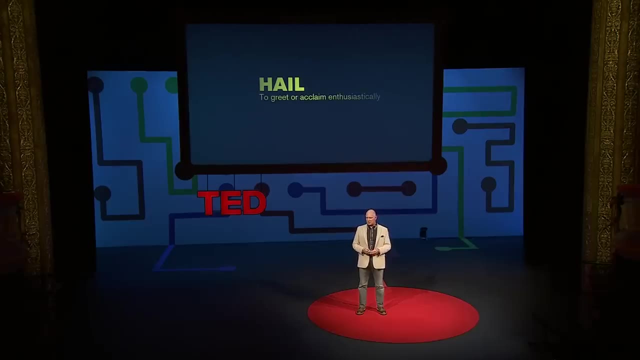 powerful and to make change in the world. Fortunately, these things spell a word. The word is hail, and it has a great definition as well. I'm not talking about the stuff that falls from the sky and hits you on the head. I'm talking about this definition: to greet or acclaim enthusiastically. 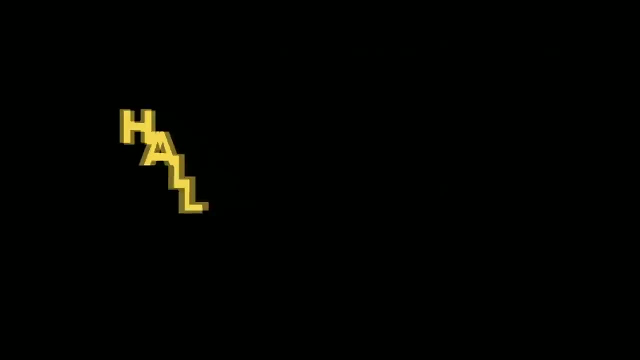 which is, I think, how our words will be received if we stand on these four things. So what do they stand for? See if you can guess: The H honesty, of course, Being true in what you say, being straight and clear. And the H honesty, of course, Being true in what you say, being straight and. 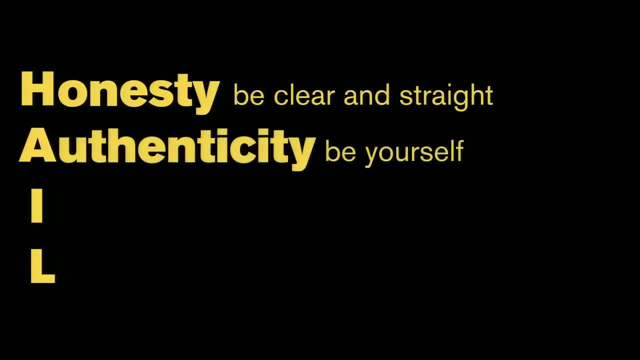 clear. And the H- honesty, of course, Being true in what you say, being straight and clear. And the The A is authenticity, just being yourself. A friend of mine described it as standing in your own truth, which I think is a lovely way to put it. 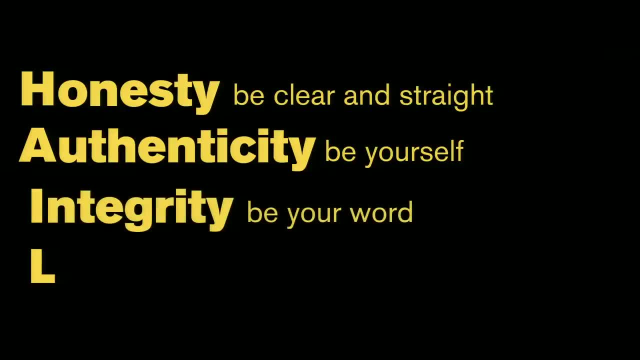 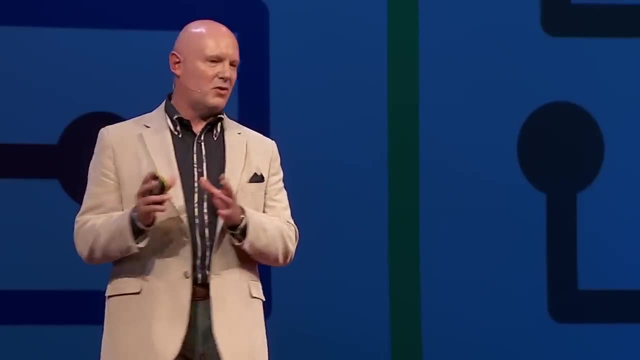 The I is integrity- being your word, actually doing what you say and being somebody people can trust- And the L is love. I don't mean romantic love, but I do mean wishing people well, For two reasons. First of all, I think absolute honesty may not be what we want. 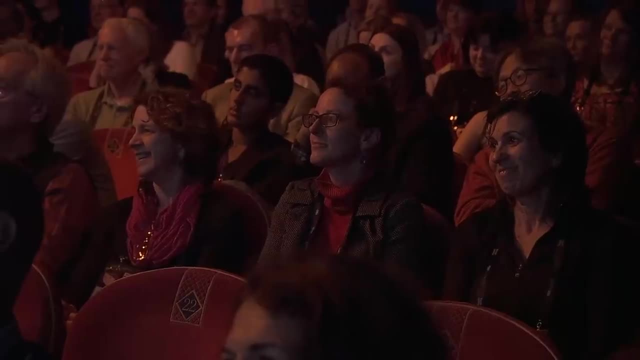 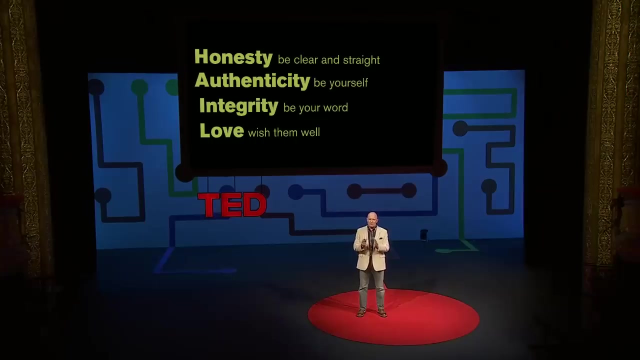 I mean, my goodness, you look ugly this morning. Perhaps that's not necessary, Tempered with love, of course, honesty is a great thing, But also, if you're really wishing somebody well, it's very hard to judge them at the same time. 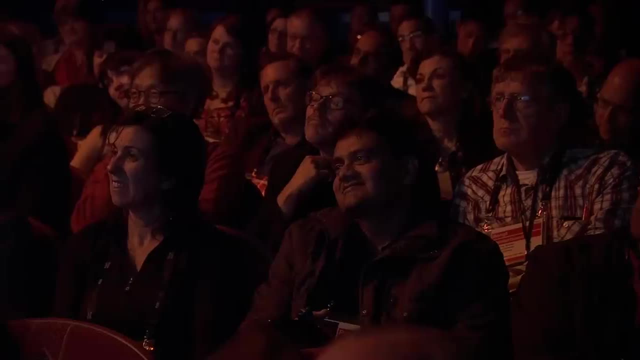 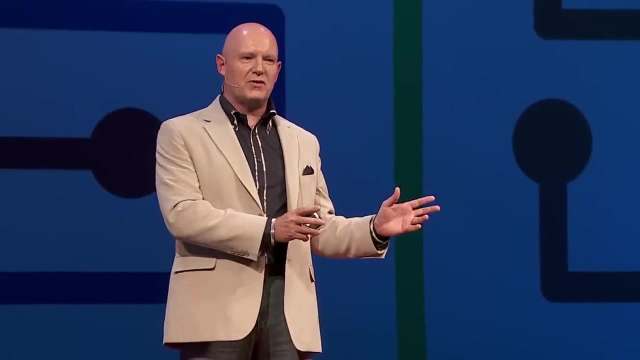 I'm not even sure you can do those two things simultaneously. So hail Also. now, that's what you say, and it's like the old song. It is what you say. It's also the way that you say it. You have an amazing toolbox. 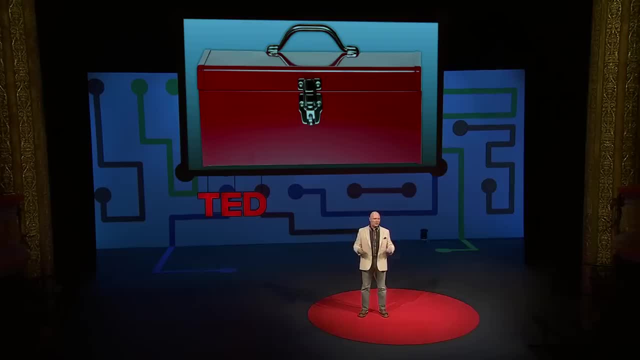 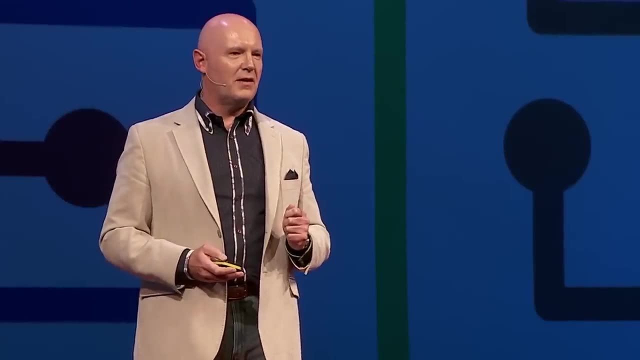 This instrument is incredible, and yet this is a toolbox that very few people, very few people, have ever opened. I'd like to have a little rummage in there with you now. Just pull a few tools out that you might like to take away and play with. 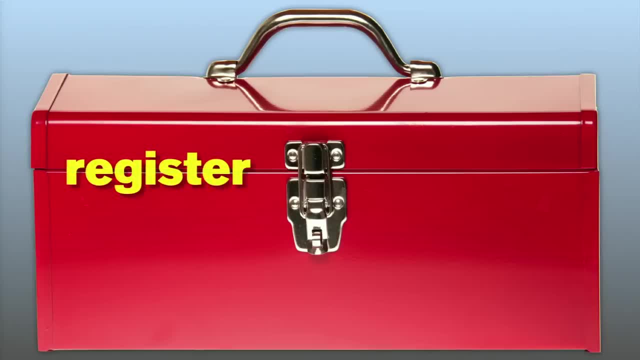 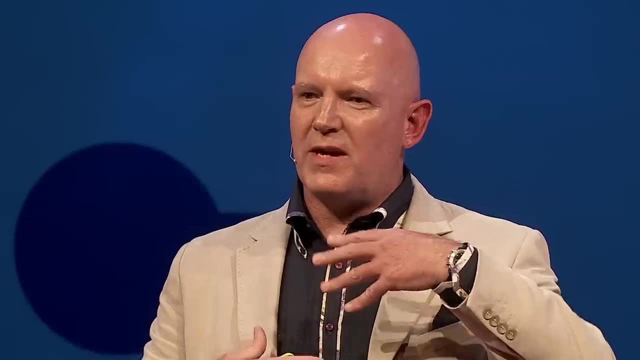 which will increase the power of your speaking Register, for example. Now, falsetto register may not be very useful most of the time, but there's a register in between. I'm not going to get very technical about this for any of you who are voice coaches. 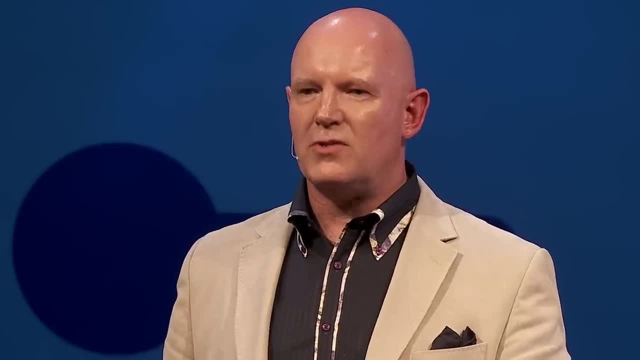 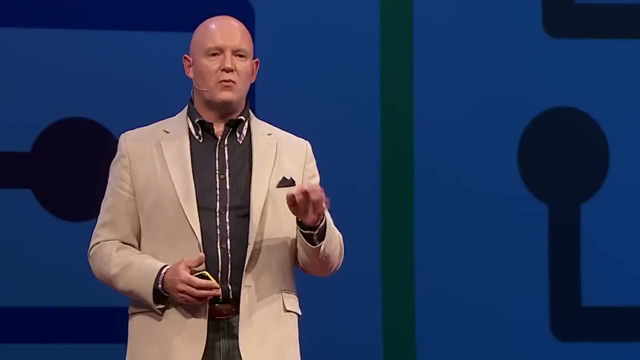 You can locate your voice, however. So if I talk up here in my nose, you can hear the difference If I go down here in my throat, which is where most of us speak from most of the time. but if you want weight, you need to go down here to the chest. 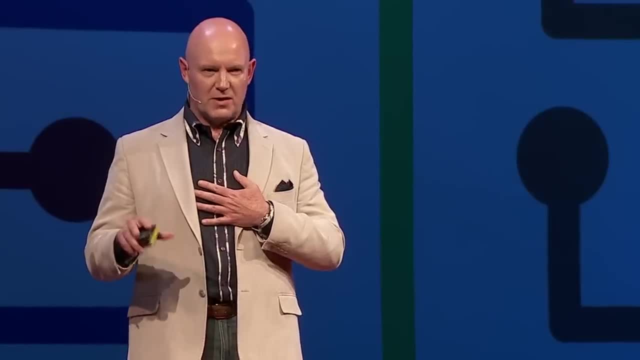 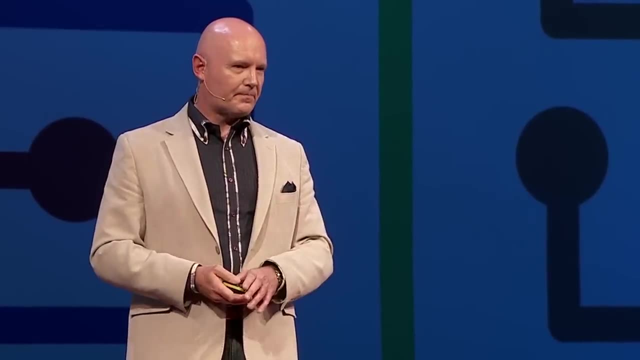 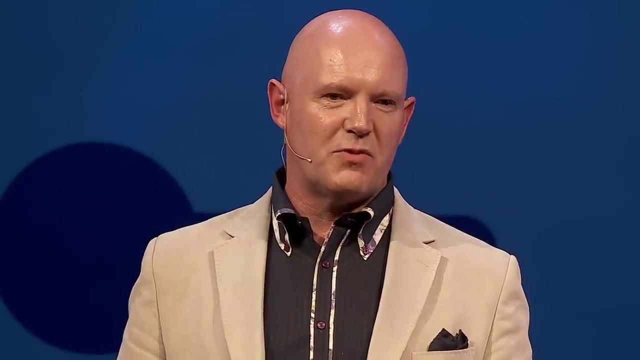 You hear the difference. We vote for politicians with lower voices. It's true, because we associate depth with power and with authority. That's register, And we have timbre. It's the way your voice feels. Again, the research shows that we prefer voices which are rich, smooth, warm. 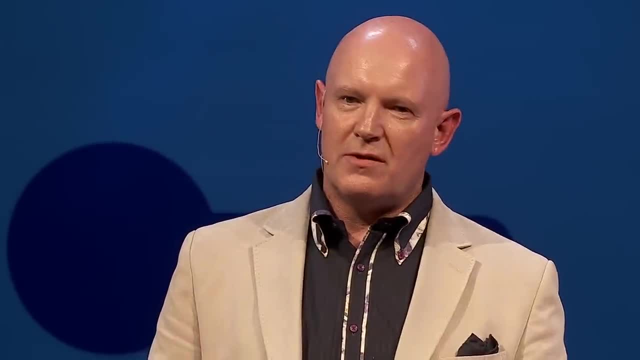 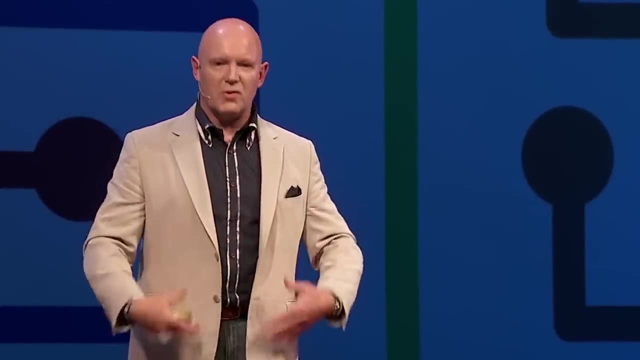 like hot chocolate. Well, if that's not you, that's not the end of the world, because you can train, go get a voice coach And there are amazing things you can do with breathing, with posture, with exercises to improve the timbre of your voice. 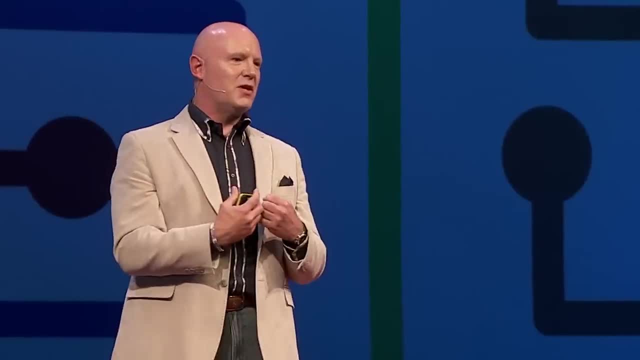 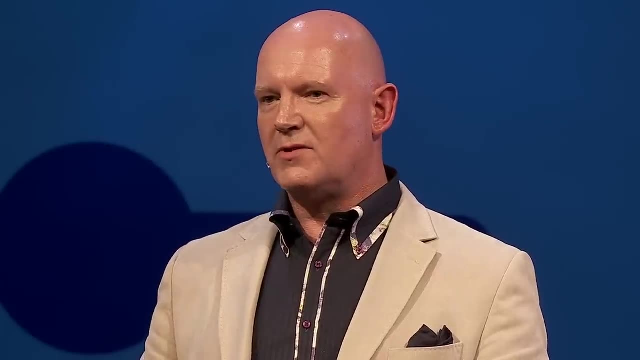 Then prosody. I love prosody. This is the sing song, the meta language that we use in order to impart meaning. It's root one for meaning in conversation. People who speak all on one note are really quite hard to listen to if they don't have any prosody at all. 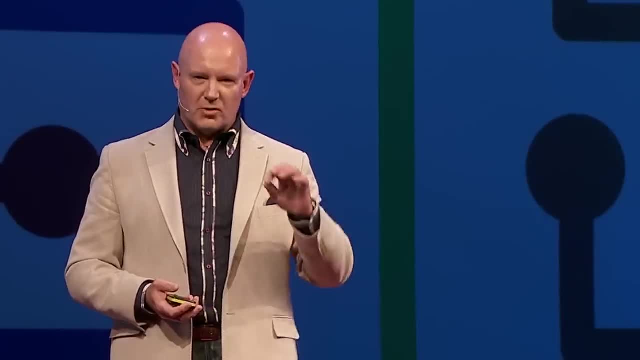 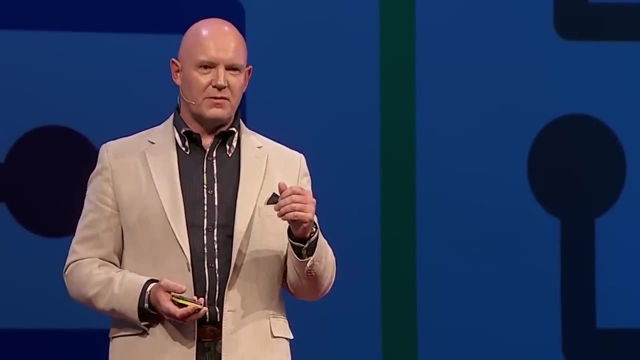 That's where the word monotonic comes from, or monotonous Monotone. Also, we have repetitive prosody now coming in, where every sentence ends as if it were a question, When it's actually not a question: it's a statement. 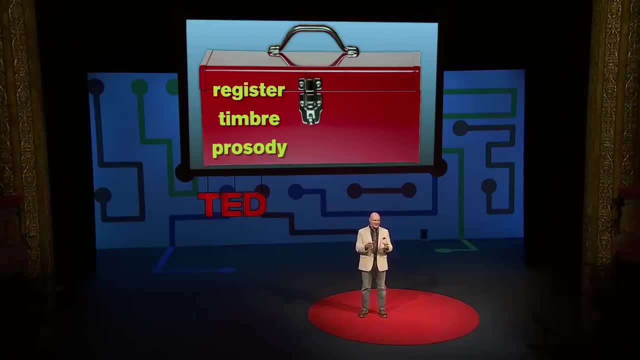 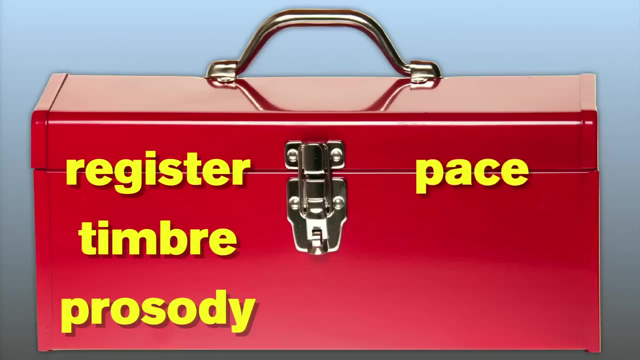 And if you repeat that one over and over, it's actually restricting your ability to communicate through prosody, which I think is a shame. So let's try and break that habit. Pace, I can get very, very excited by saying something really, really quickly. 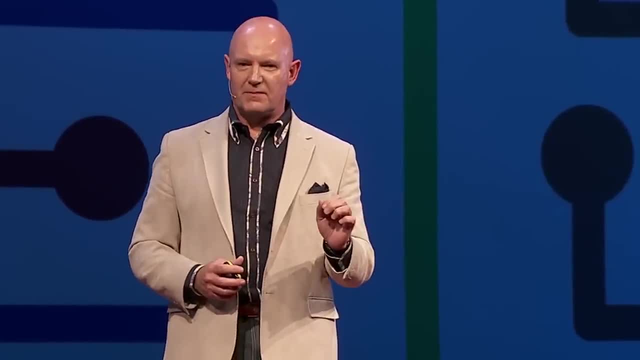 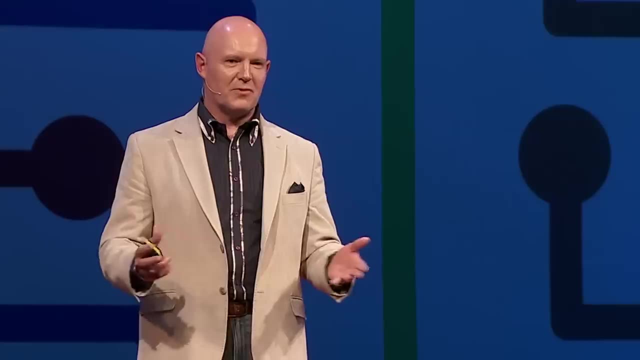 or I can slow right down to emphasize, I can slow right down to emphasize, I can slow right down to emphasize, And at the end of that, of course, is our old friend silence. There's nothing wrong with a bit of silence in a talk, is there? 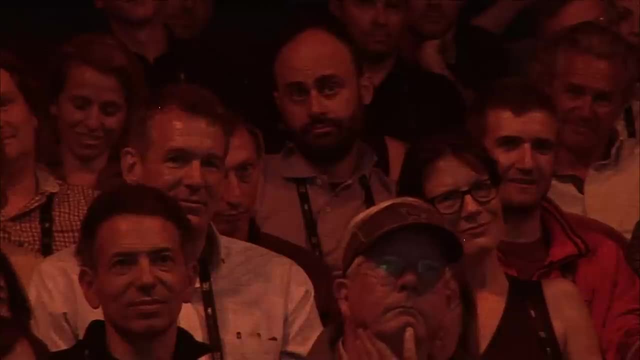 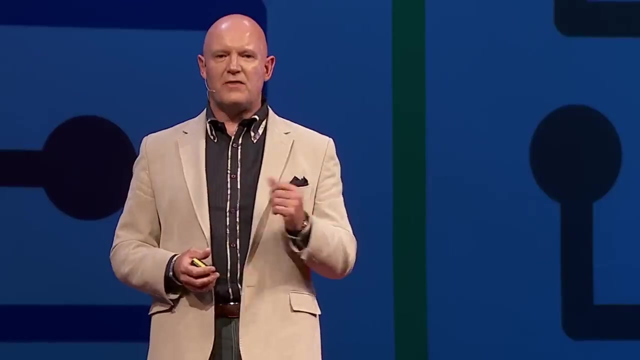 We don't have to fill it with ums and ahs. It can be very powerful. Of course, pitch often goes along with pace to indicate arousal, but you can do it just with pitch. Where did you leave my keys? Where did you leave my keys? 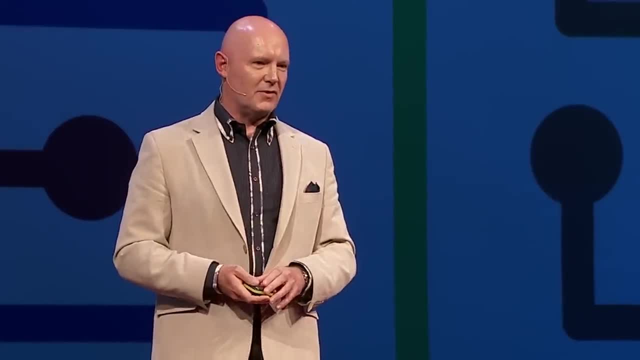 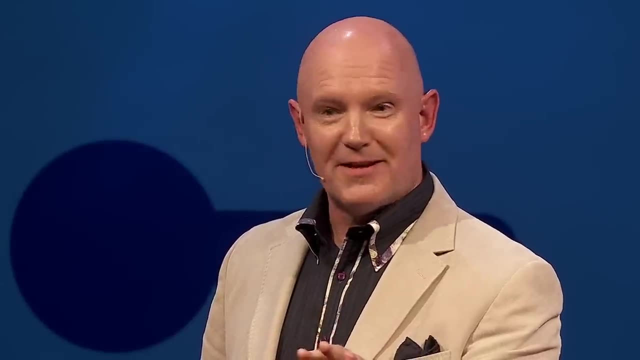 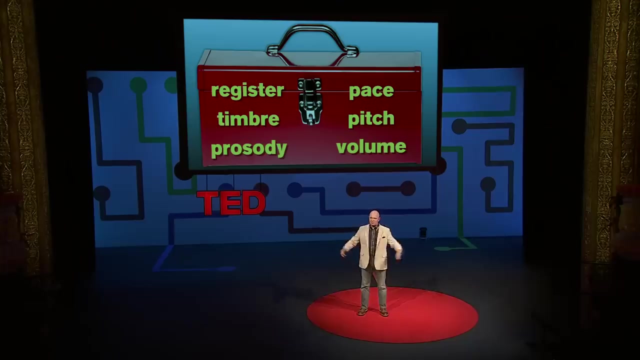 It's a slightly different meaning in those two deliveries. And finally, volume. I can get really excited by reusing volume- Sorry about that if I startled anybody- Or I can have you really pay attention by getting very quiet. Some people broadcast the whole time. 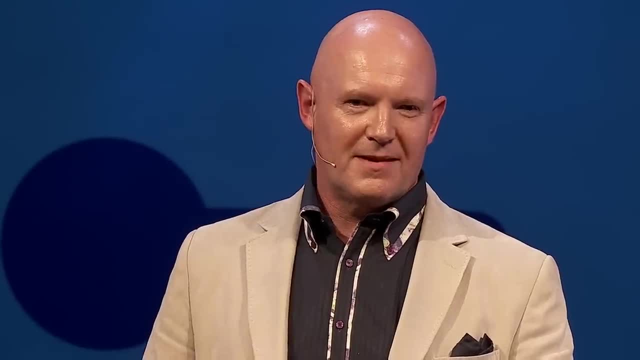 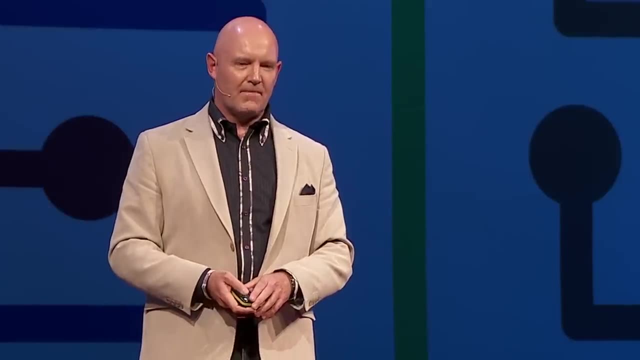 Try not to do that. That's called sodcasting- Imposing your sound on people around you carelessly and inconsiderately- Not nice, Of course. where this all comes into play most of all is when you've got something really important to do. 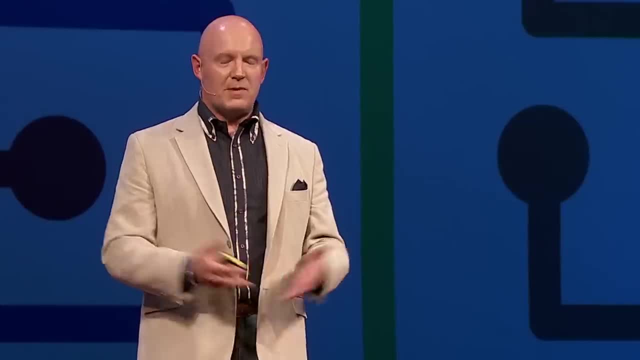 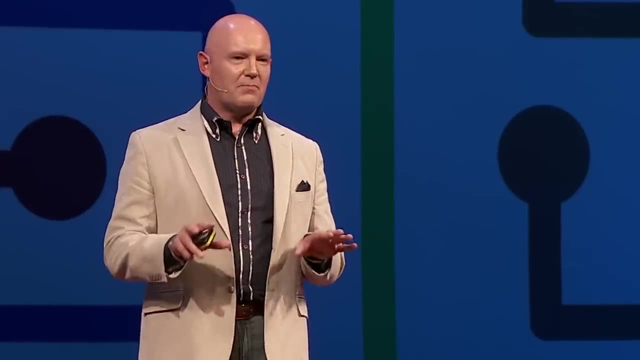 It might be standing on a stage Like this And giving a talk to people. It might be proposing marriage, Asking for a raise, A wedding speech. Whatever it is, If it's really important, you owe it to yourself to look at this toolbox and the engine that it's going to work on. 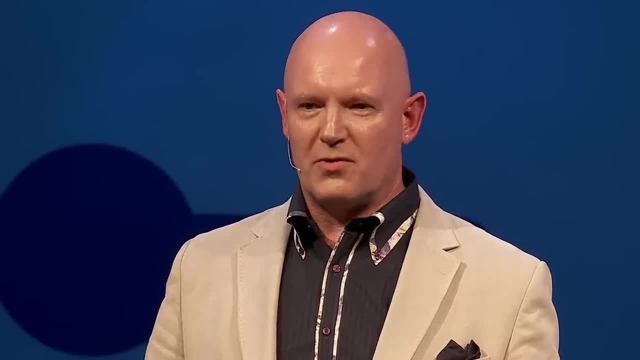 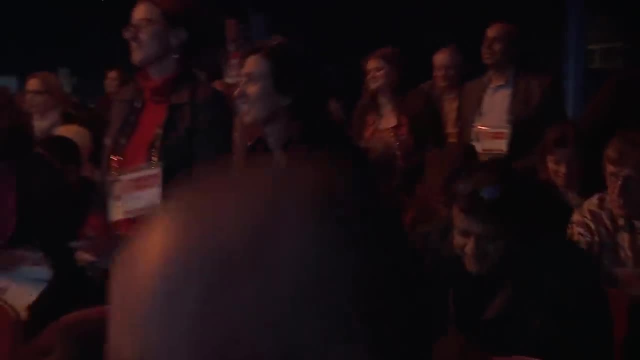 And no engine works well without being warmed up. Warm up your voice, Actually. let me show you how to do that. Would you all like to stand up for a moment? I'm going to show you the six vocal warm-up exercises that I do.